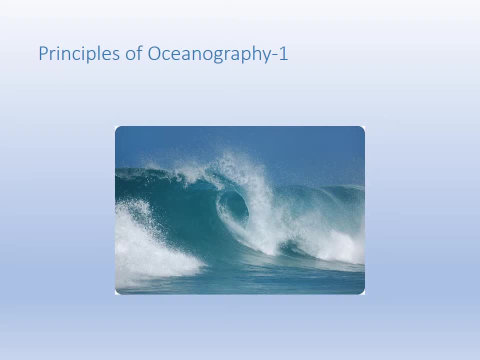 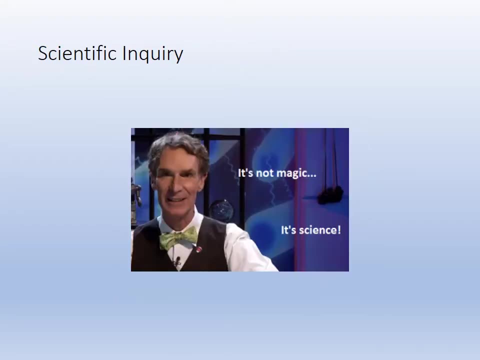 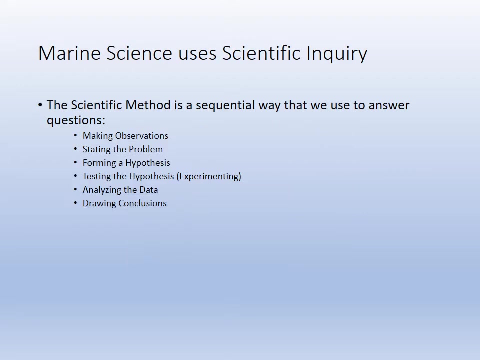 I'd like to welcome you all to the first lecture of Marine Biology OCB. So we'll start off with scientific inquiry. You can see Bill Nye, a contemporary of Bill Nye. Most science classes start off with a scientific method. Scientific method is a sequential way used to answer. 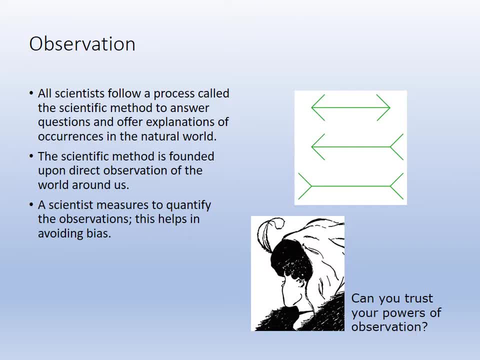 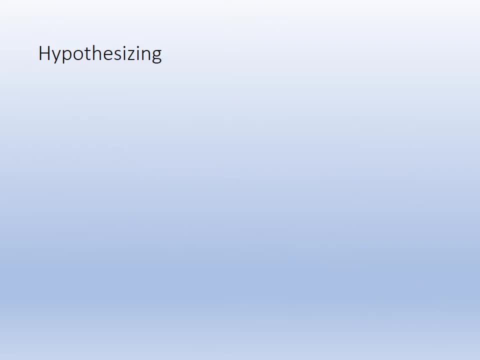 questions. This slide shows you how your powers of observation, which may be the most important step. Hypotheses are statements that explain observations. We test them with the experiment Experiments. you have a control group which is lacking what you're testing. 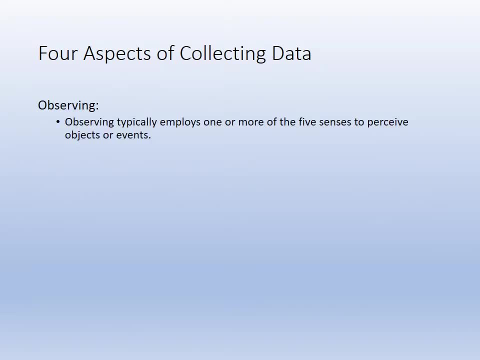 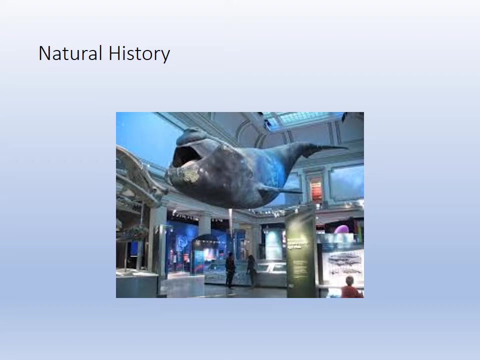 It forms the baseline. Observing is your first aspect of collecting Data. Your conclusions give you a new model, allow you to infer on. The next topic, so to speak, is the natural history of the ocean. There's- we'll start off approximately 14. 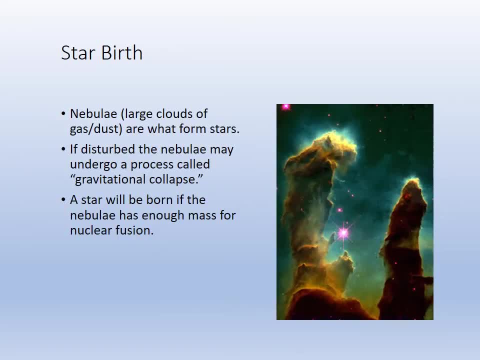 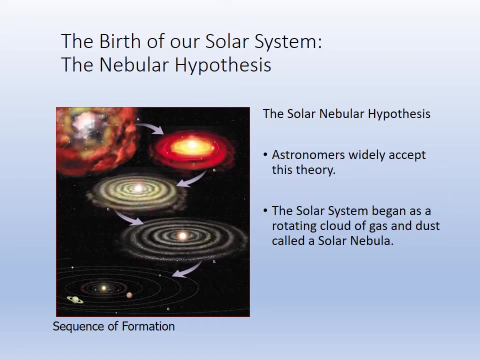 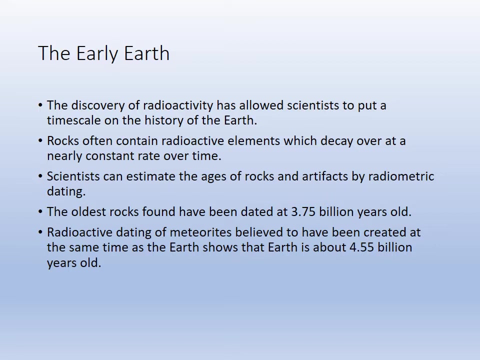 billion years ago, 13.5, 13.. So stars are born in these gas clouds, generally Hydrogen, called nebula. They collapse with. We call that the nebular hypothesis. So our early Earth. early Earth, Condensation, collision accretion. So the early Earth. 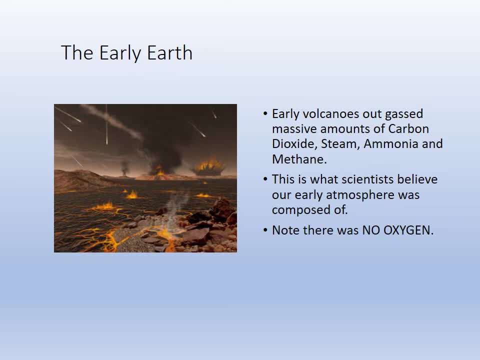 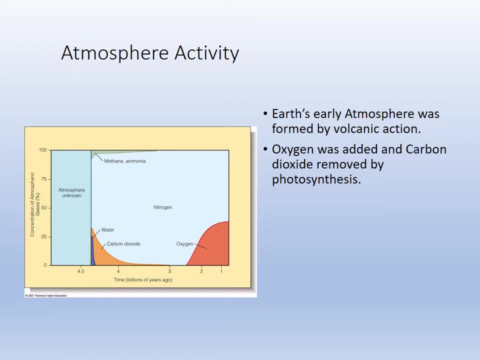 No oxygen in the atmosphere. We can tell that there was no evidence. So our early atmosphere, So our early Earth. So our early Earth. So our early Earth, You can see, unknown in the beginning, as we were cooling, Condensing, So oceans outgassed. 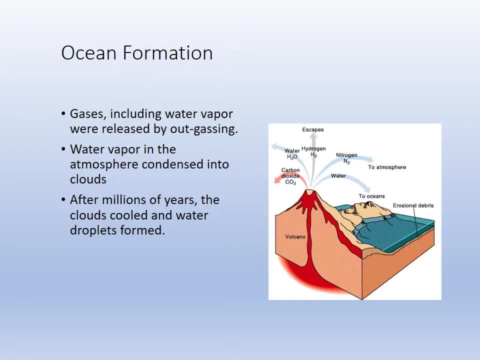 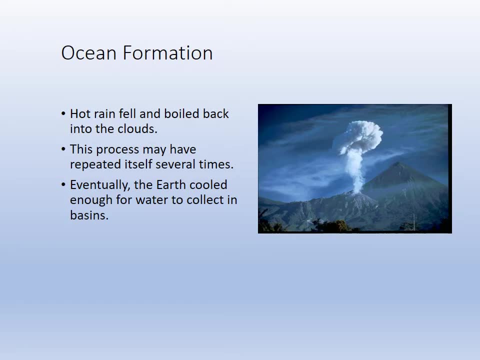 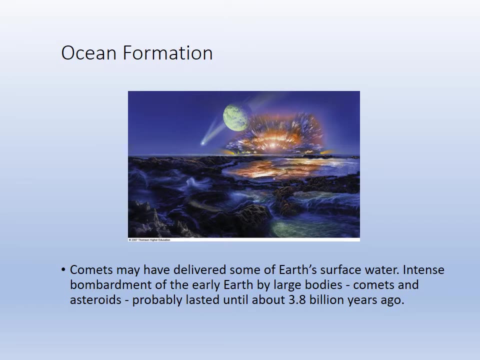 Some probably from comets, but most of it outgassing. You know, the rain falls, boils falls. Earth stabilizes in that first three quarter We have. we're sweeping out of orbit. So we have a lot of meteorite impacts The moon without. 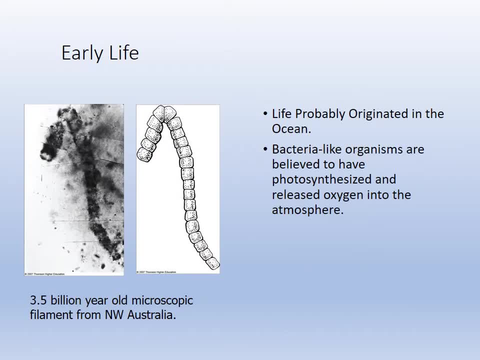 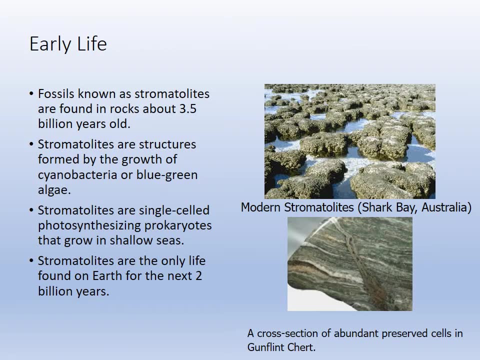 So we have a lot of meteorites impacts The moon without Early life. were microscopes- Microscope most likely in our tidal zone because we didn't have that oxygen. Our033 00118- There's modern tomato likes. You can see how they're layered with oxidation. That's a reaction with oxygen. 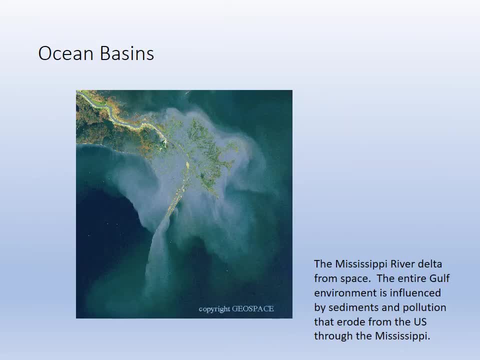 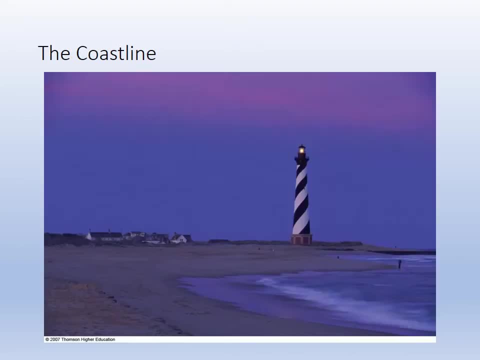 So our first oxygen showing up. Now we're going to skip to the ocean basins. Let's just get a handle. We'll start with the coast. That's what we're going to do. the bulk of our studying is is the climate. 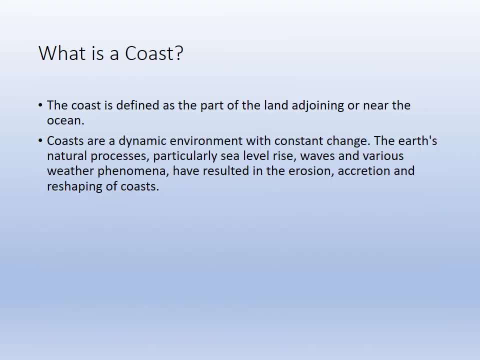 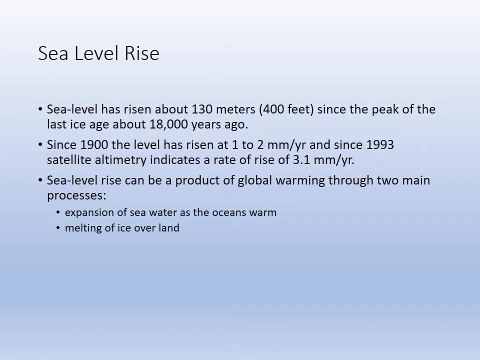 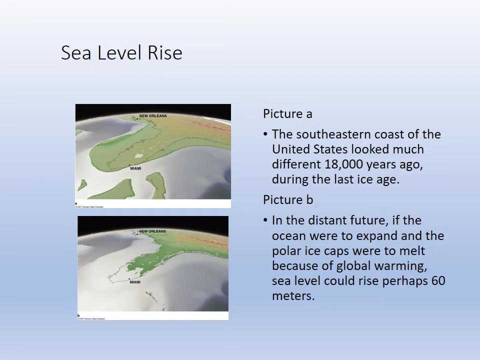 coast, west coast of florida. so coast is the part of the land adjoining the ocean. it's dynamic, which means it's always changing. sea, uh, sea level currently is rising. sea levels rising uh, the glaciers melted by 18, so sea level rises. the first image was 18 000 years ago. that's our continental. 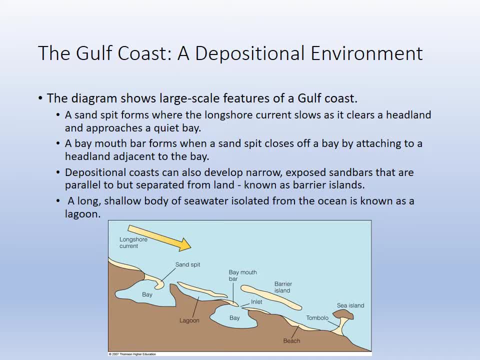 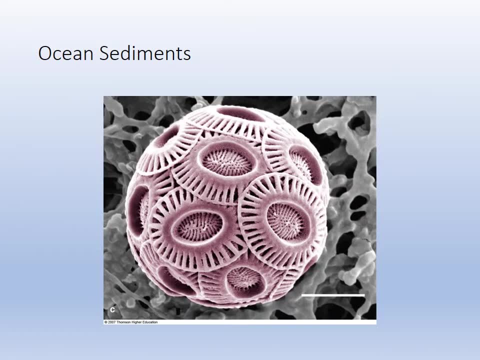 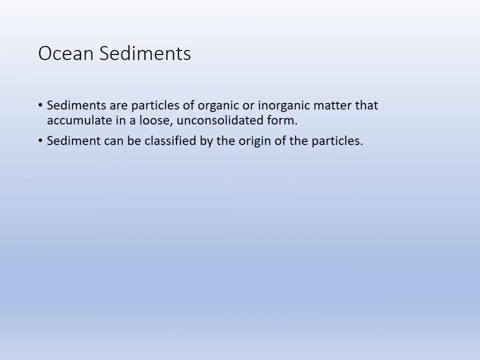 margin. uh, we live on a depositional coast. depositional coast is typified by barrier islands. you can see a little bit uh. this ocean floor is covered with sediments. a picture uh right there is of uh, so sediments on are loose. some organic organics are called oozes. 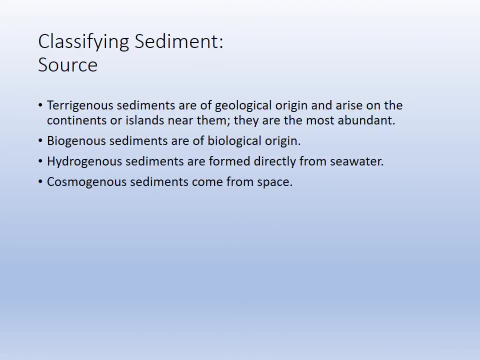 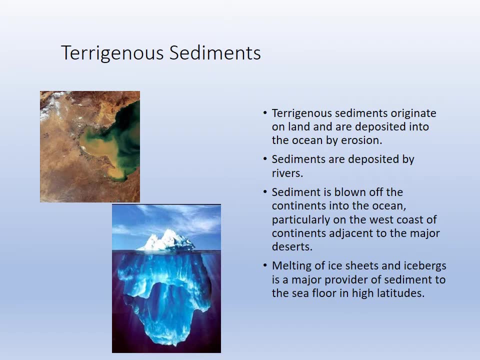 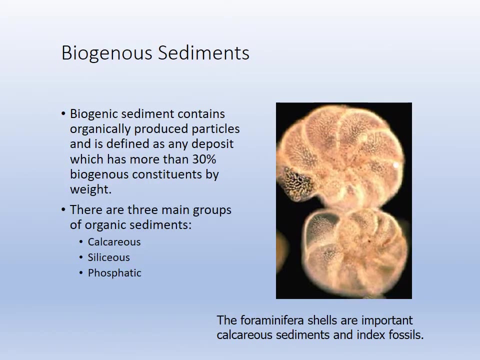 so, uh, we have terra genius, land-based biogenius, that's our plankton, that when they die, they're skeleton. so there's some images of terra genius: uh, weathering and erosion, glaciers, biogenius, sediment is the plankton that falls. it literally rains. in quotation marks down. 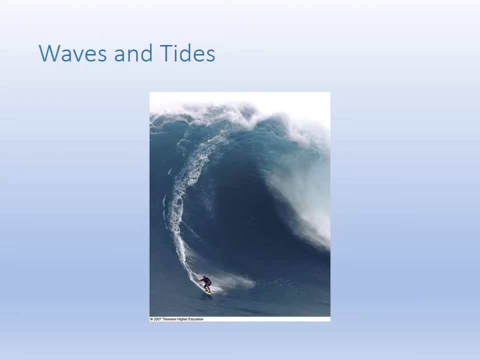 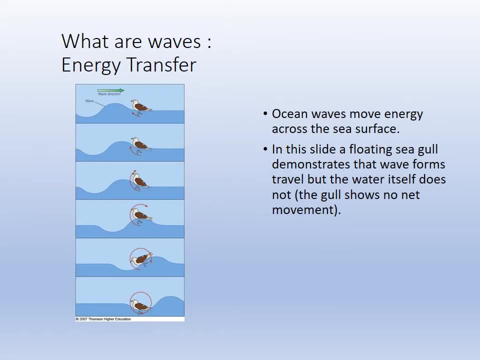 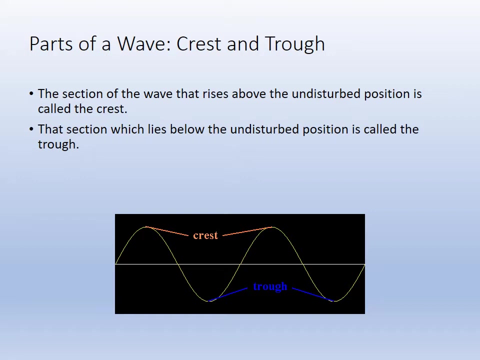 uh, looking at the waves and the tides, some physical aspects of the marine environment. uh, waves are energy transfer, so they're going across the surface. uh, the crest is the high point of the wave and the trough is the low point. the amplitude is how high that crest or how low that trough is. 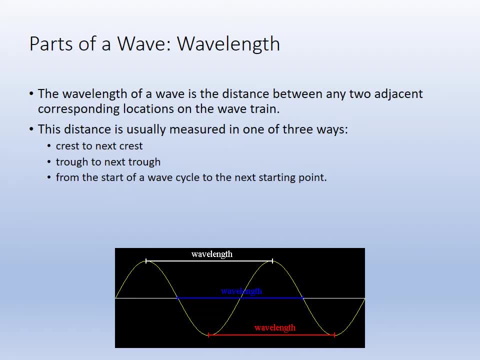 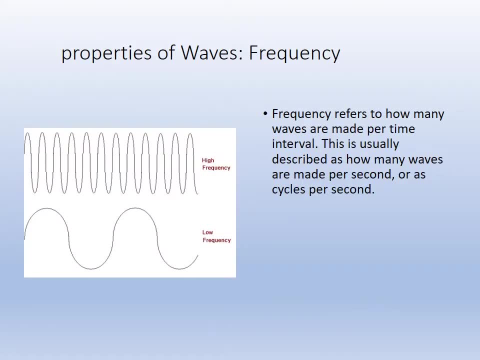 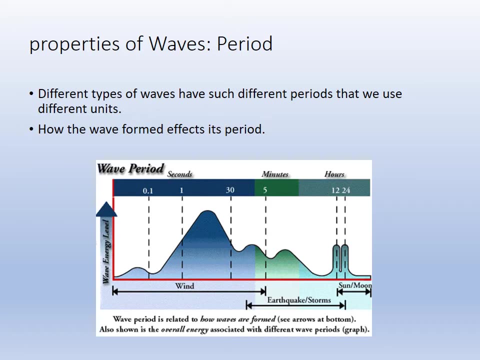 the wavelength is the difference between two successive waves, so it's the length of one wave, so that's how many waves are passing by, and so the frequency is how many waves per second pass by. so a higher frequency or a lower frequency, and we're discussing this because of this image. 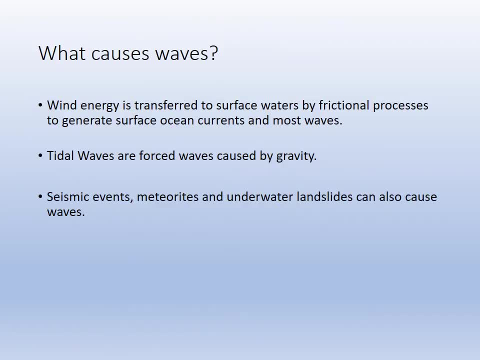 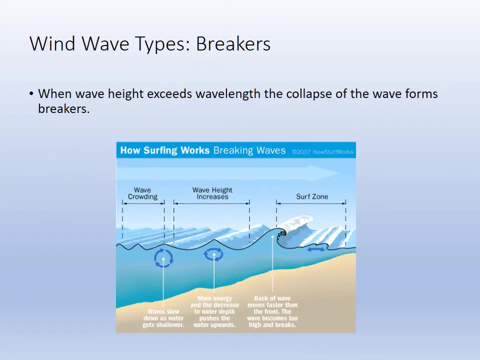 here you can see wind waves. wind waves are the most common. it's what we deal with every day. so waves are caused by the wind, gravity, tides between the sun and the moon, and when they reach half of their wavelength. So waves are undisturbed. We. 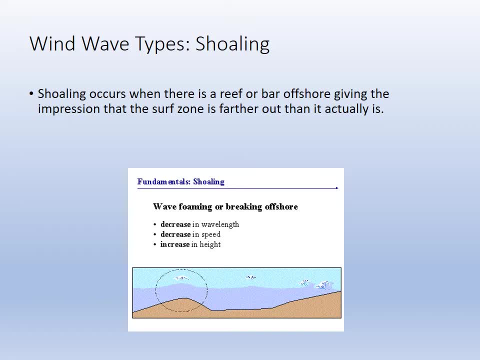 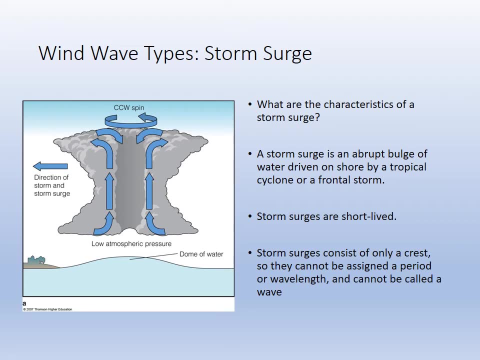 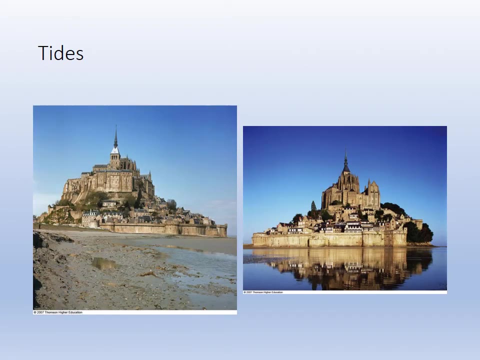 call the breaking of a wave an area shoaling. so waves break or shoal in that surf zone Half a wave storm surge. Storm surges are short-lived Speaking of tides, there's Mont Saint-Michel in France and that is an extreme example of a high 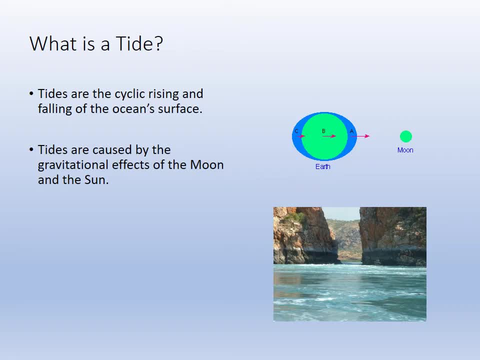 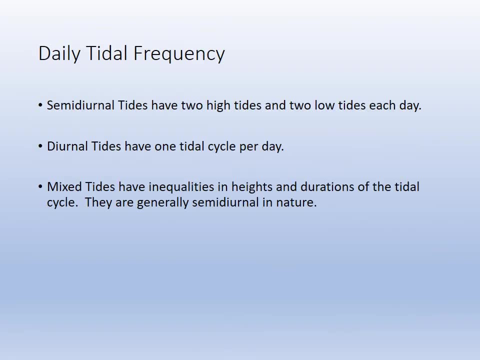 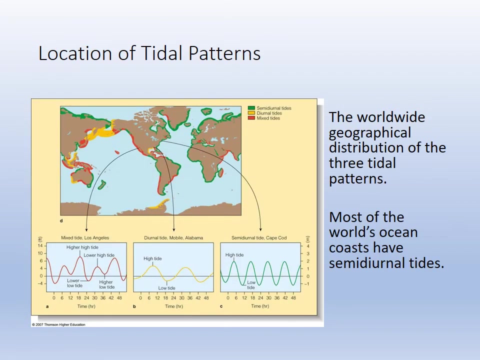 tide, low tide. There's two tidal bulges on Earth at all times. One's caused by the moon's gravity, one's So semi-diurnal and diurnal. Here, here in our area, we have a mix, which means most. So this map shows you where on Earth each tidal cycle. 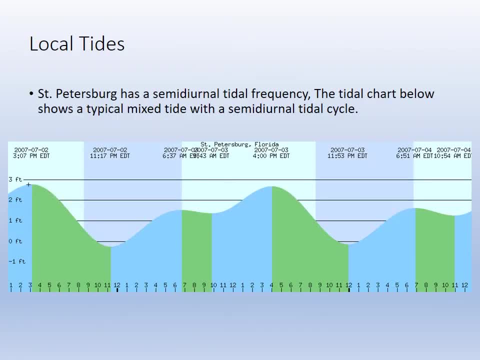 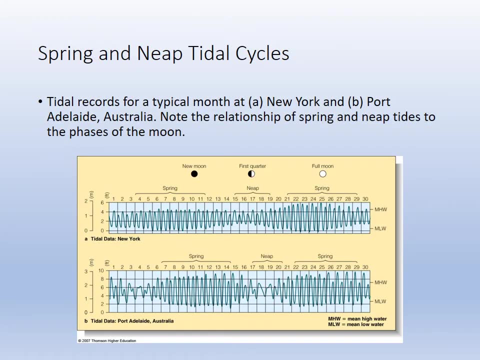 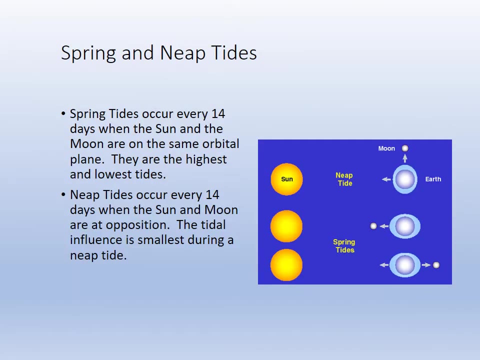 occurs. There's just a local semi diurnal mix. This shows you your spring and neap, Very important in the marine environment. When you have a salt marsh, the, So it's all lunar phase. You can see when the neap tide you're at a quarter phase, So temperature changes. 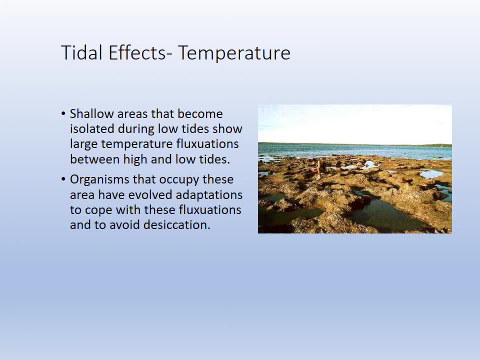 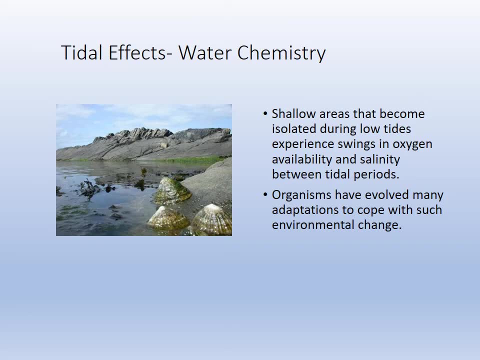 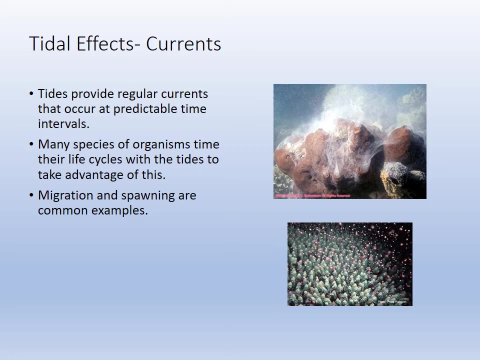 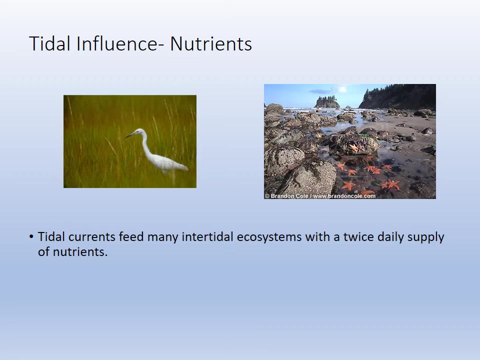 every day There's some tide pools, high tide, new water comes in, So it changes the chemistry as well. Organisms, as I said, reproduce on the tidal cycle, So you have a picture of a. Tides bring the nutrients into and out of their ecosystems. Your salt marshes your tidal.